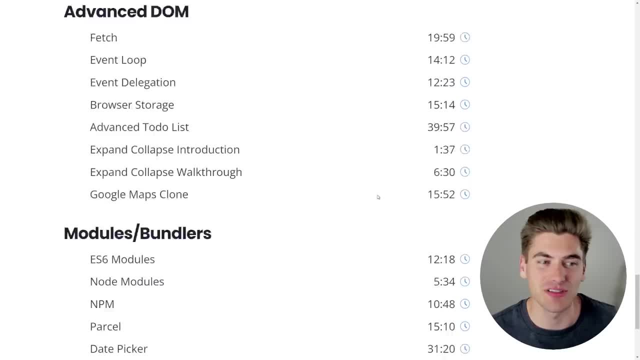 so you can start building your dream project sooner. You'll notice we have this massive list of topics we're going to cover in this video. This right here is only half of the things that we're going to cover, and you'll also notice that this is actually coming from. 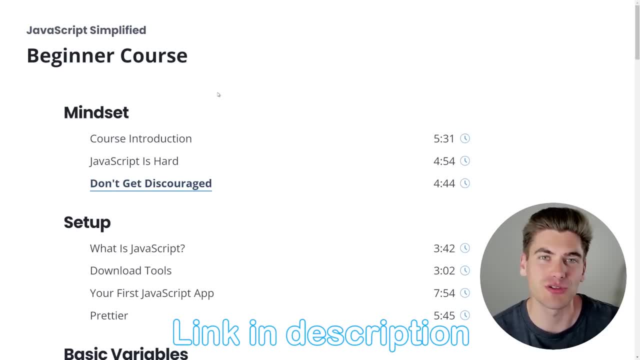 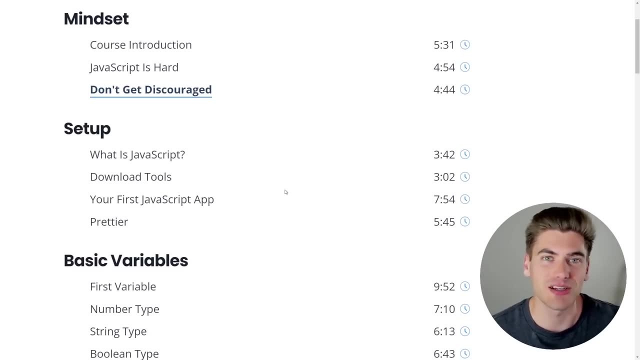 my JavaScript Simplified course. I'm going to put a link down to the course in the description, as well as this table of contents. So if you're interested in learning JavaScript, you can go ahead and take my course, and it's going to cover every single one of these topics in order. 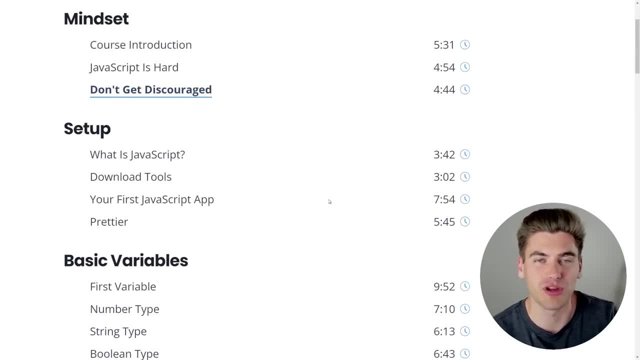 exactly, But, like I said, you can go and find these topics online for free on YouTube or blog articles and so on. This is just meant to be a way of explaining what order you should learn things in, in my opinion. So the very first thing I want to talk about is how you set up your 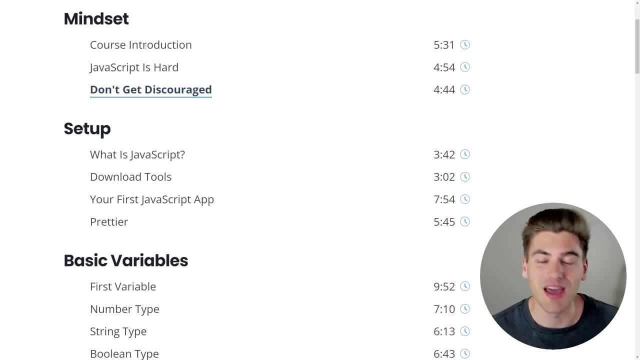 mindset for learning these topics. This is something almost everyone skips, and it's really important to actually set your mindset correctly to make sure you're in the right mindset for learning JavaScript. Like I mentioned at the beginning of this video, it's very difficult to. 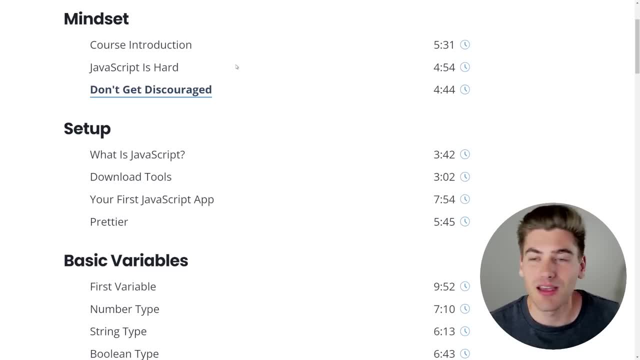 learn JavaScript, so you need to make sure you go in understanding that And I'd recommend actually watching this. Don't Get Discouraged video. If you just click this link right here, it'll bring you directly to that video. You can watch it completely for free, no issues. You don't have to sign up for. 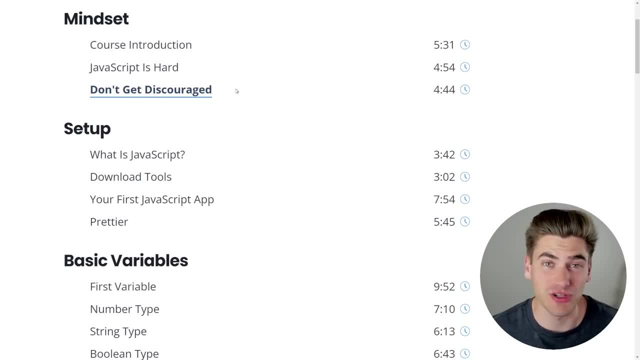 anything. You just click it. it'll play the video for you. I recommend watching that before you start learning JavaScript, just because it will really help you get in that mindset that you need and not get discouraged by struggles or things that you run into. So once you've got that done, 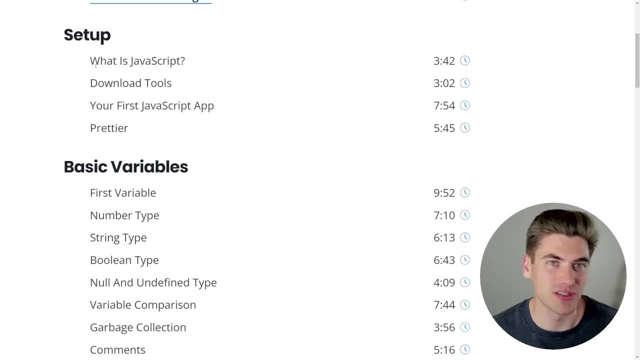 the next step is obviously setup. Luckily, with JavaScript it's really easy. You just need a web browser and a textbook to set up your mindset. for learning JavaScript, You just need a web browser and a text editor. I recommend Chrome and VS Code. That's what I use, but really you can use whatever. 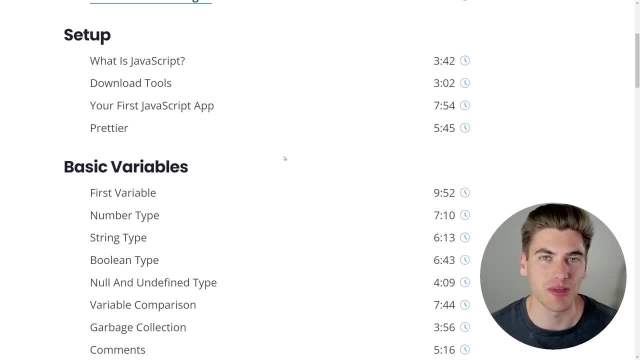 you want, Then also, I use Prettier inside of JavaScript. It makes formatting code a little bit easier. I have a full video covering that. It's completely free on YouTube. I'll link it in the cards and description for you. So if you want to use Prettier for your formatting, like I, 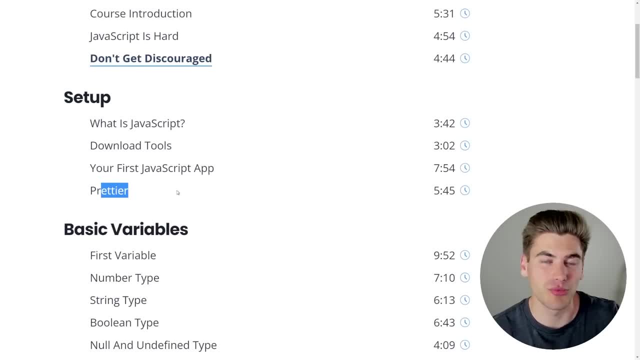 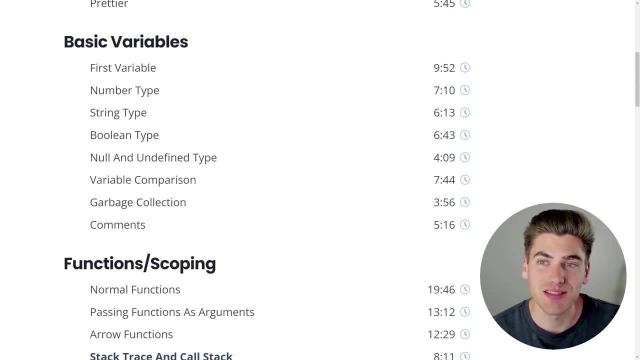 recommend that'd be like the next step And that right there takes care of all- like the preview steps- all the things you need to do in order to get started working with JavaScript. Luckily, it's a pretty small list of things Now. once you've got all that set up, the very first thing- 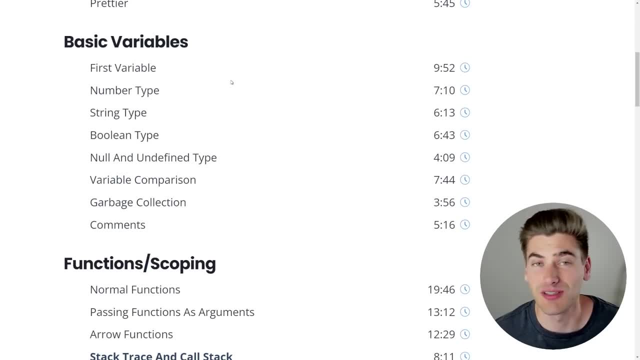 that you're going to want to learn is going to be variables inside of JavaScript. This is how you store information in JavaScript, and this includes things like numbers, strings, booleans, null, undefined, and so on. So I really only want you to focus on the basic variables. 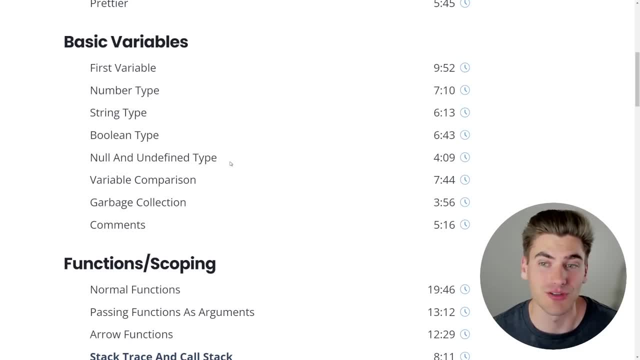 these types right here that are listed. There's only five different types and they're very easy to understand and learn. Just learn what they are. learn how you can set variables and change variables. That's going to be what you care about here. Then, at the end here, you'll notice I have a 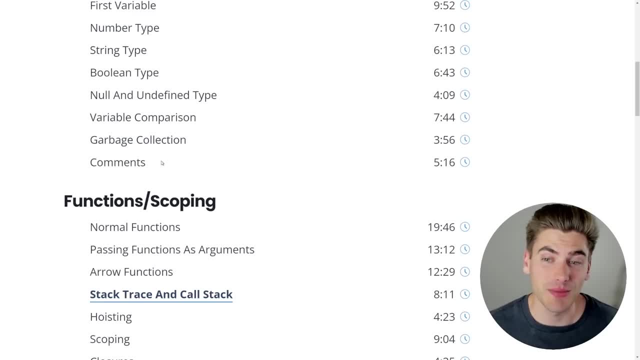 video on garbage collection, as well as comments. It's important to learn how to write comments in JavaScript, and also garbage collection is important, just understanding how that works. You can just Google it, read a quick article or watch a video on it. It's pretty straightforward. 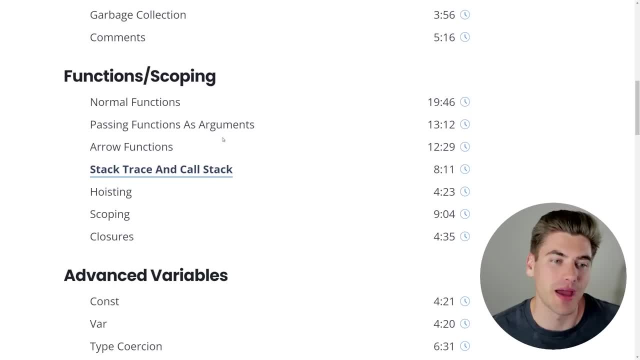 and simple. If you want to learn how to write comments in JavaScript, you can just google it. and not something you actively need to think about, It just happens in the background. Now, the next thing to learn, once you've learned variables, is to learn functions and how scoping. 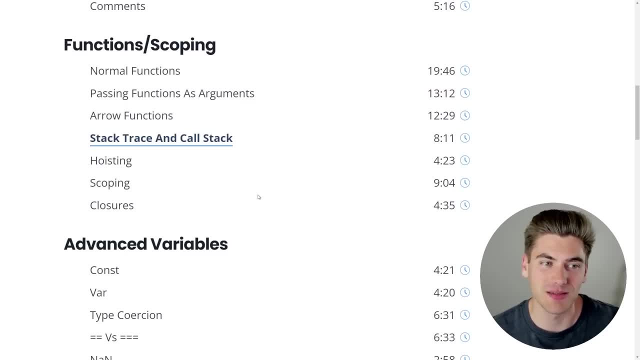 works in JavaScript. This is one of the most important basic concepts that you're going to understand These different concepts right here: how normal functions work, how hoisting works, how scoping works and how closures work. These are some of the core, fundamental concepts to how 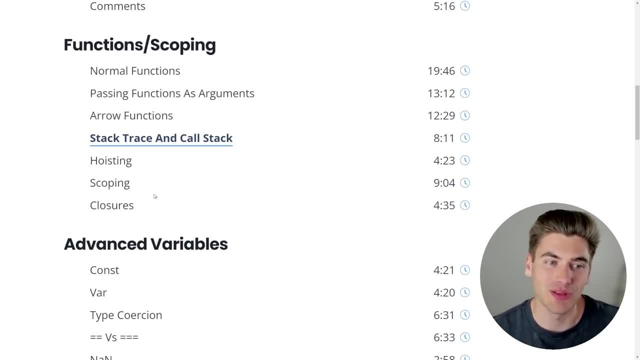 the entirety of JavaScript works, so I really recommend spending lots of time focusing on these different topics and really understanding how they work and how they actually interact with each other. This is going to be a lot of fun and it's going to be a lot of fun and it's going to be a 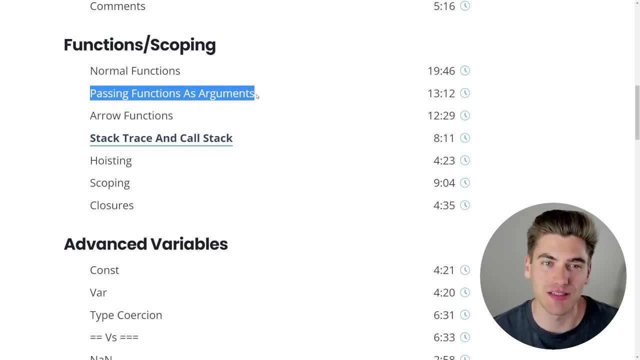 lot of fun. This is going to be one of the biggest bang for your bucks that you can get. as well as this, passing functions as arguments video. I again have a video covering this right here for free. I'll link it in the cards and description for you. 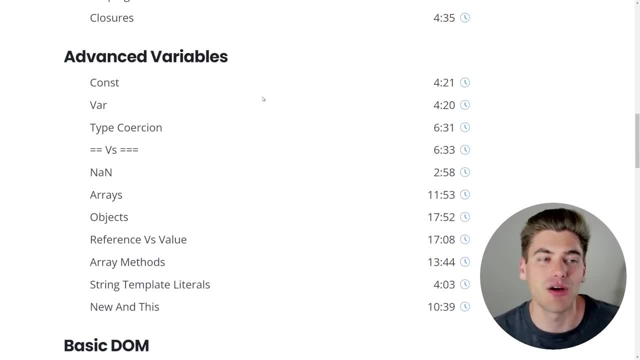 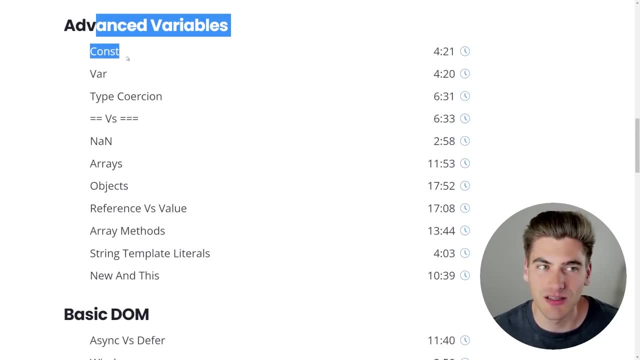 but understanding those concepts is incredibly important. Now, if we move on here, you see we have an advanced variables section. It just expands upon this basic variables section by talking about things like const and var and other things like that, like how the different equal signs work. 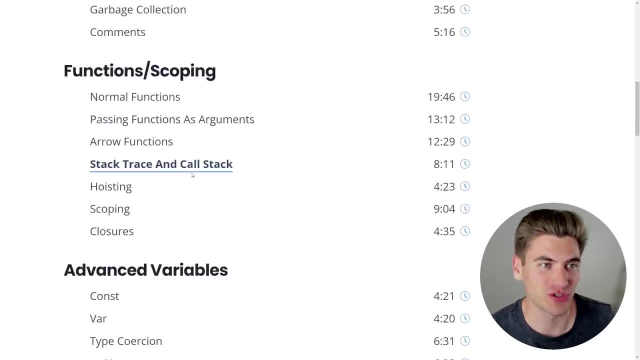 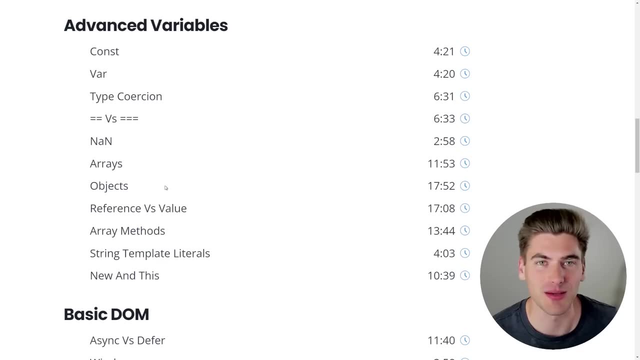 This, again, is one of the really important building blocks to learning JavaScript. just like with functions, Understanding things like objects is crucial, because almost everything that you deal with in JavaScript is going to deal with objects in some way, which is again why reference versus value is really important. I also have a free video on. 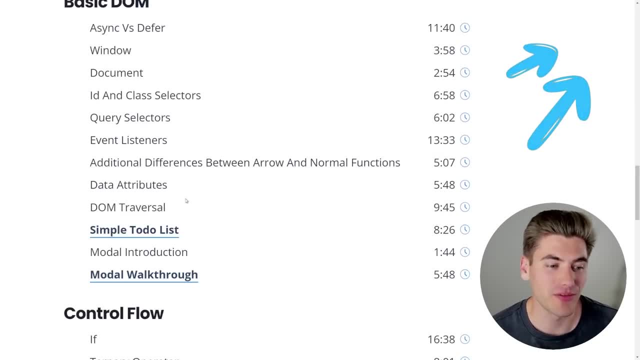 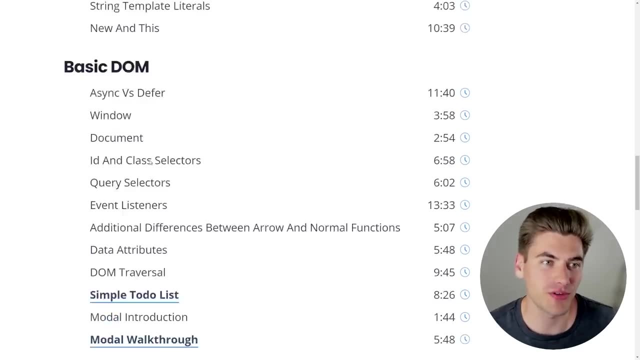 that I'll link it in the cards and description for you. Now, moving on, we have this really large section here, and this is just covering the very basics of interacting with the DOM, and the DOM is just like a web page. So far, everything we've covered up to this point. 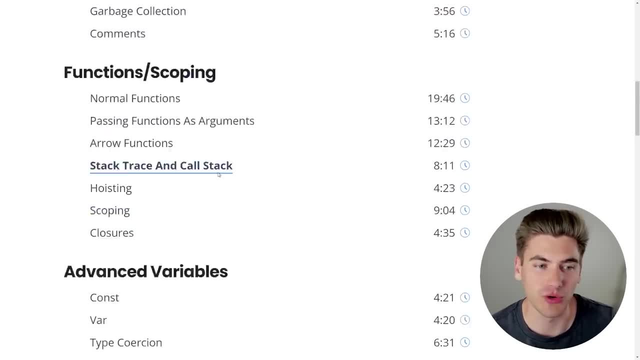 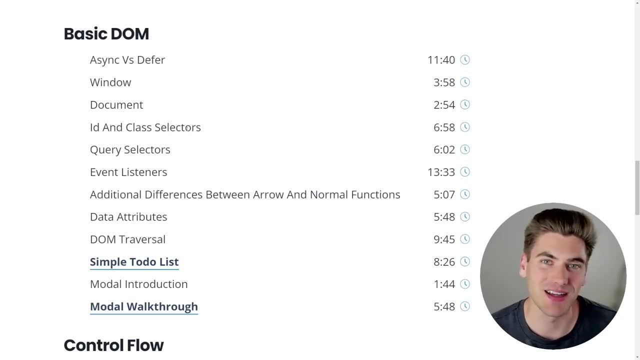 all of this has nothing to do with web development. It's JavaScript only. The DOM is the only web development specific thing that we learn about JavaScript. so this is just covering the most basic concepts of the DOM. This is just covering the most basic concepts of the DOM. 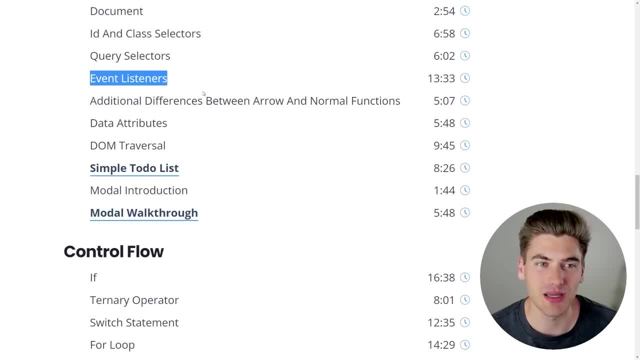 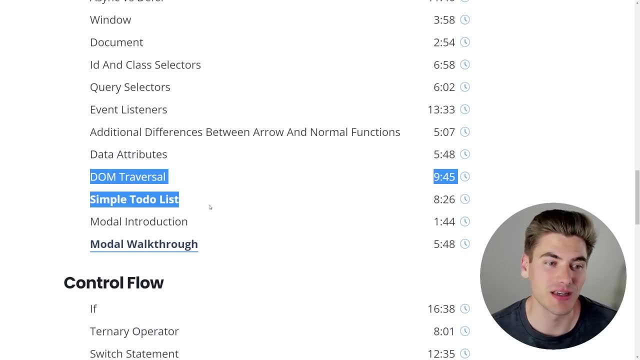 like: what is the document, how do you select different elements, how do you set up event listeners, like when you click a button, how do you do something, and some other really simple concepts like that. And, most importantly, this is where we start to get into some of the very 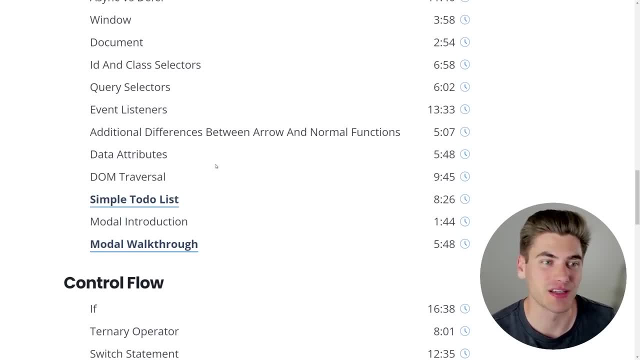 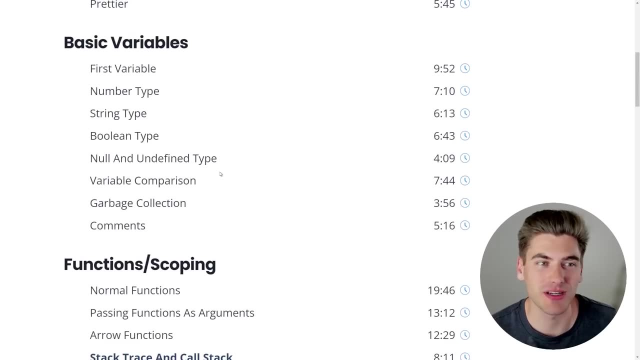 first projects in my course and most likely in your learning journey as well. Up until this point, the concepts we've been learning have all been building blocks to build on top of each other in order to do something with JavaScript, because you can't really build a project if all you know. 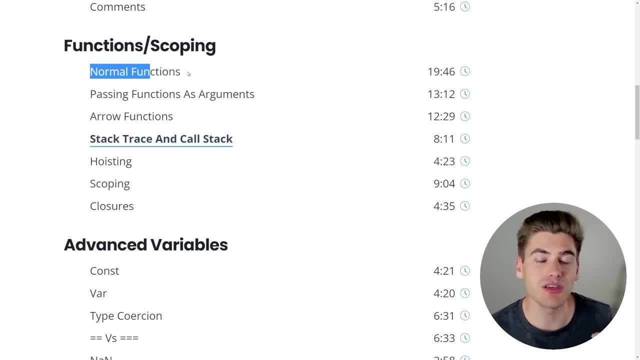 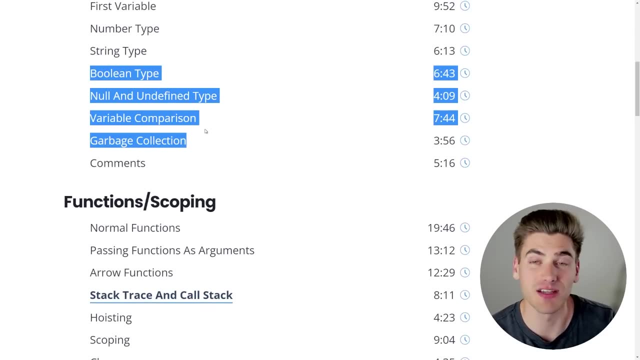 how to do is create a number variable or create a function. You need to be able to interact with something and you can practice these concepts and I highly recommend you to do so. I highly recommend practicing these concepts, like in all of these videos in my course we have tons of. 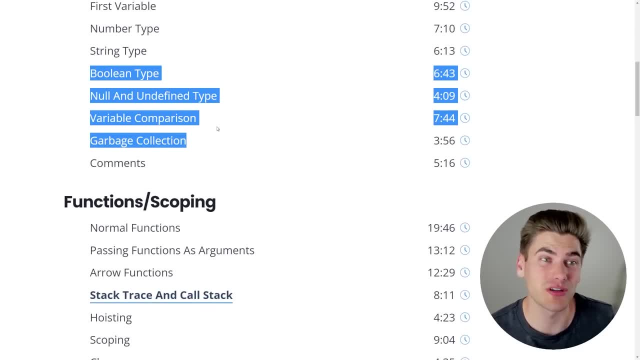 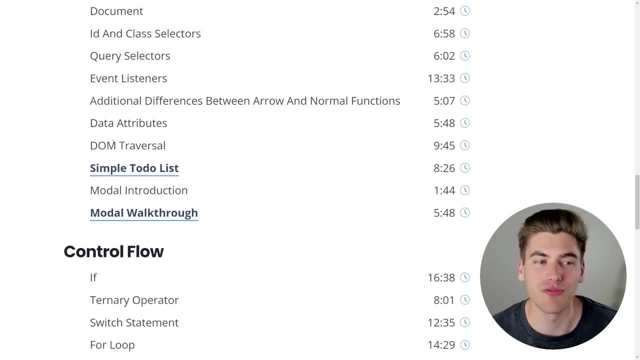 exercises in the video to practice these concepts. but, like I said, it's really hard to build some type of project because we have no way to interact with the web or the DOM. That's why, when we get to the basic DOM here, this is where we have the very first few projects coming in As 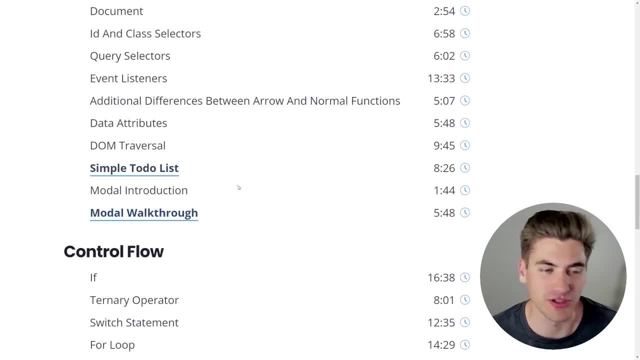 you can see, you can actually watch these videos on the first two projects of the course. if you want. you can just click on these links. it'll show you the different projects. So I would recommend, with a very basic project, This simple to-do list. here is a super basic to-do list. 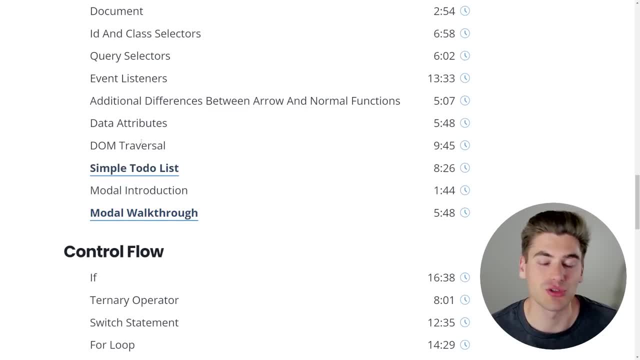 project. same thing with this model. As you can see, they're less than 10 minutes long, so don't start with anything super crazy when you start doing your first project. just make it really small and simple, just to try to implement the different concepts. 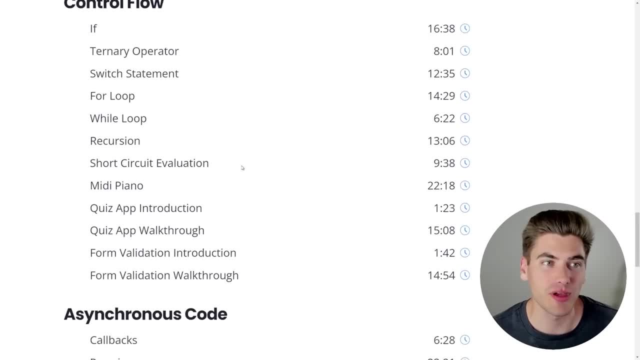 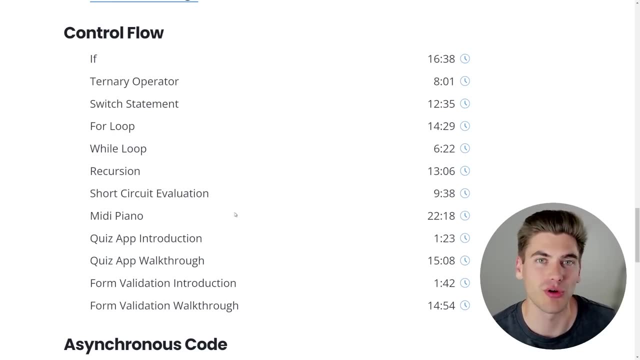 you've been learning up to this point about the DOM. Now, moving on from there, we get into control flow. This is another one of those building block concepts which is super important, and this is how you do anything logical in your program. So far, everything we've done just runs. 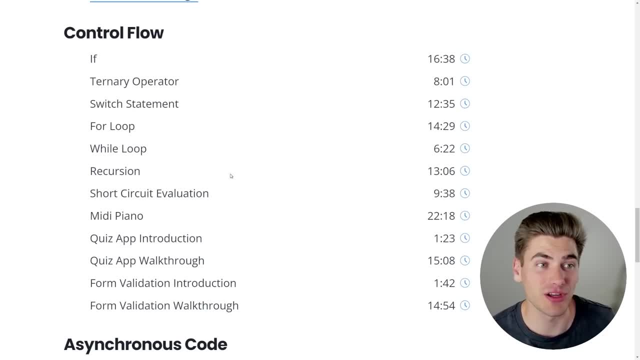 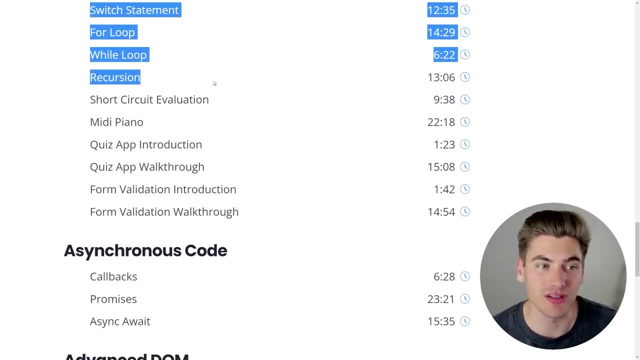 top to bottom and it just executes once and that's it. At this point in the control flow we have things like if logic reverse, like if this is true, then do something else. Same thing here we have for loops while loops, so we can loop through different things. 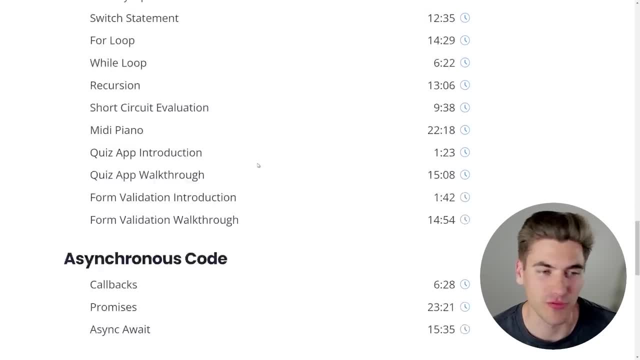 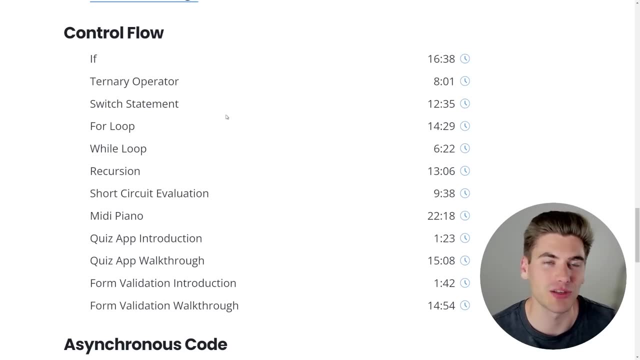 and we have a bunch of different projects. You can see at the end here we just have like three or four different projects at the very end of this section to really hammer home all those different concepts because, like I said, this control flow is a really important building block you need to. 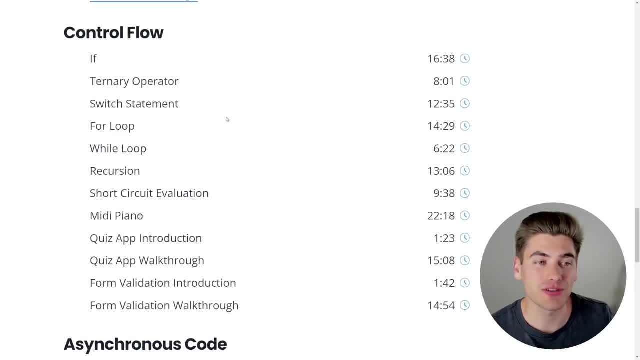 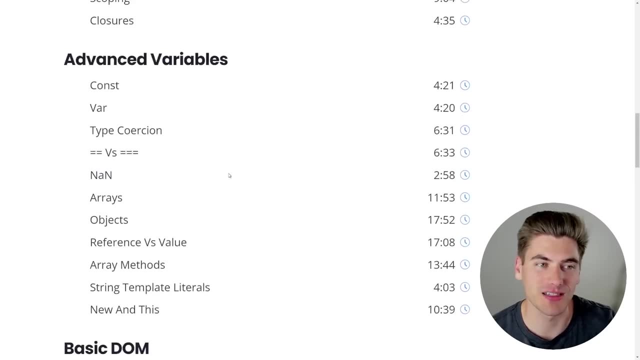 build upon. You'll notice in this course and in this roadmap that there's not a lot of projects at the very beginning. Instead, we're focusing on the really core building block concepts because, if you understand, all of these different concepts we've talked about so far at a really 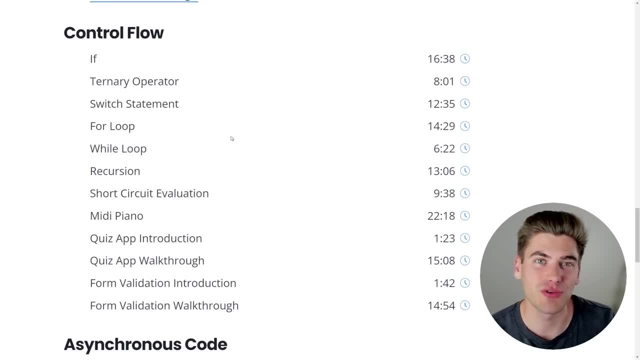 good understanding and level. that's going to make it so much easier for you to build out projects in the future and really understand what JavaScript is at the core. Because the biggest thing that people run into as a problem when learning JavaScript is you focus on following a lot of tutorials that build out really cool projects. 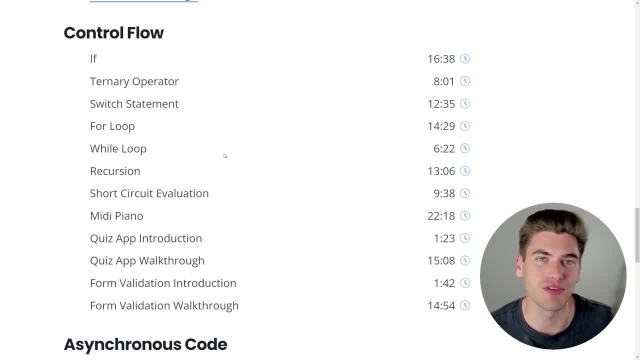 but you never actually learn the underlying concepts of how everything fits together and why it works. That's what I try to focus on in this course and in this roadmap, which is why I highly recommend focusing on those basic concepts, like I've mentioned Now. moving on from there, we get to some of the more advanced concepts in this beginner section. 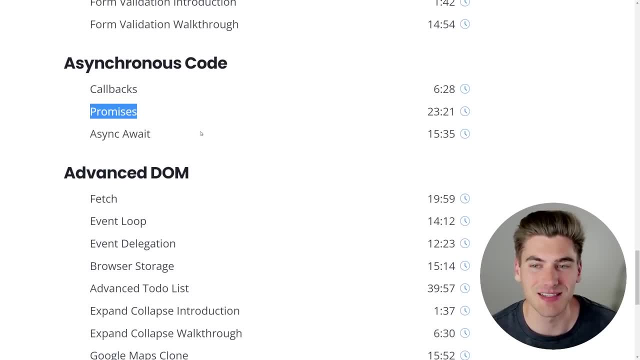 here We're talking about asynchronous code, things like callbacks, promises, async await. These are really important concepts, so I highly recommend spending your time making sure you understand these concepts when you get here, but don't skip to this section, Don't you know? 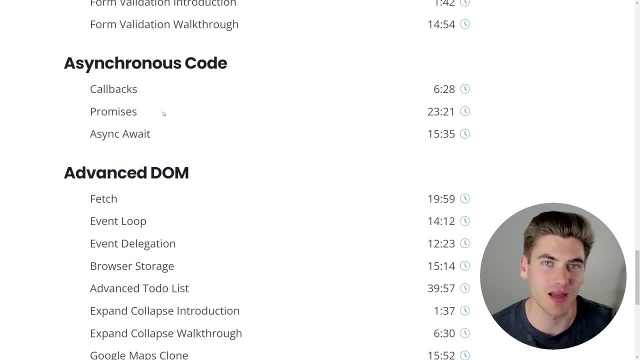 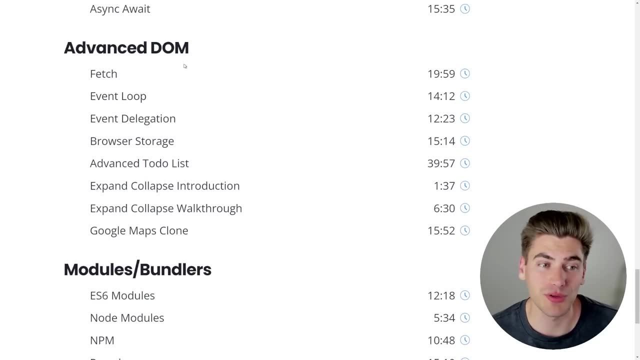 skip all the way ahead here to try to figure out what's going on. Make sure you take your time, build out the foundation and then get to these when you do, and it'll make it much easier to learn these. Now, moving on a little further, we have more DOM-related concepts. This is just 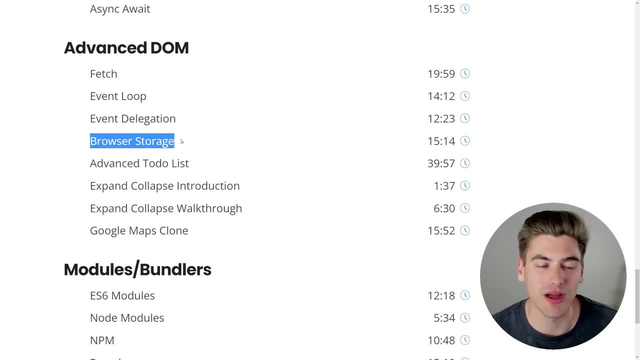 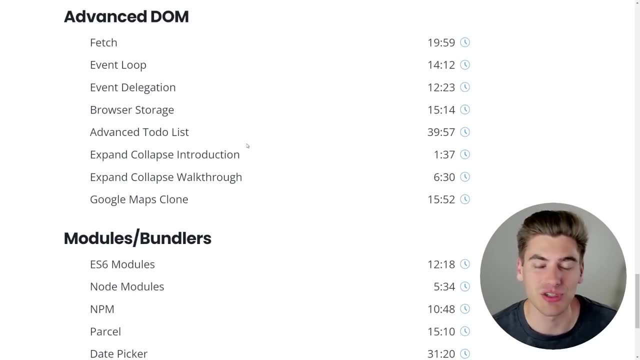 slightly more advanced things like how do you fetch from an API, how do you interact with local storage, and building out some more advanced concepts like a Google Maps clone, a more advanced to-list, that kind of stuff. So this is really focusing on some of the more advanced features. 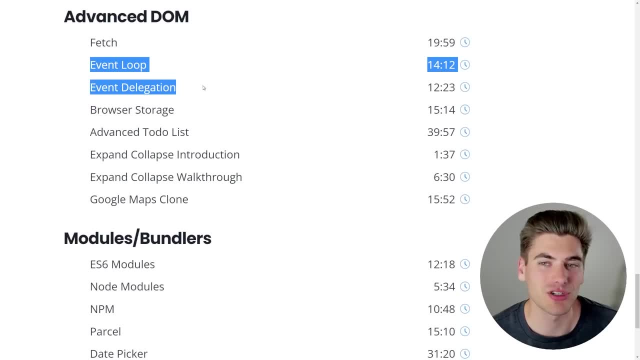 of the DOM. One of the most important here is the event loop and event delegation. Understanding how events work in the DOM is really crucial to actually working with the DOM. so these videos right here in particular are very important concepts to understand. Now the last section I want to talk about in this beginner section. 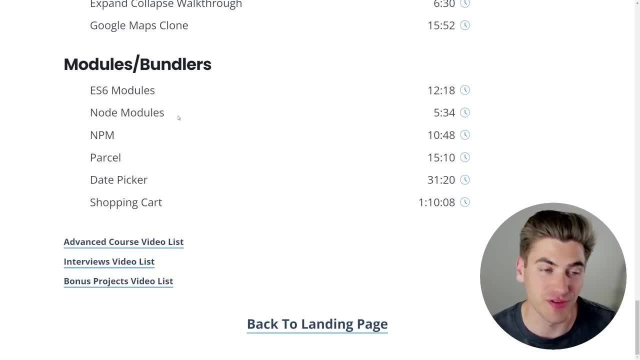 this kind of gets you to the point of a junior developer. This is actually more than I even knew when I landed my first dev job as a JavaScript developer- and that's going to be bundlers and modules. So we're talking about ES6 modules, how node modules works, as well as things like npm. 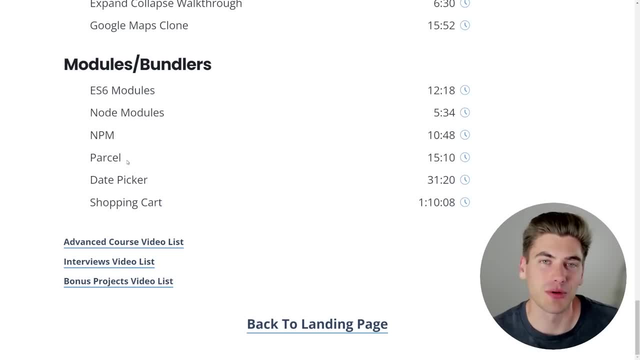 parcel, which is a bundler. Personally, I would recommend using Vite instead of Parcel. I just like it a lot better. I find it works a lot better, but you can use any bundler you want. Now, the most important thing, though, is, at this point you have a really good understanding of 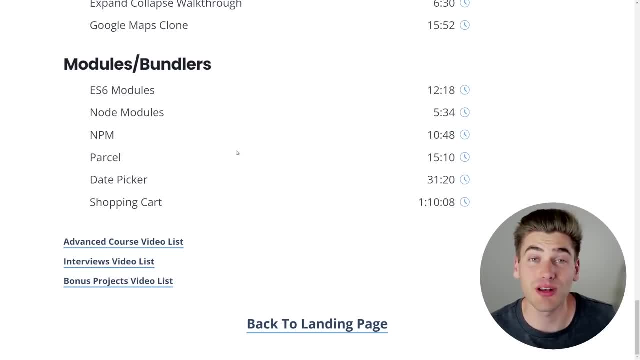 the basics and somewhat intermediate concepts of JavaScript so you can actually build out some really advanced projects. So in our case we're building out like a custom date picker as well as a shopping cart. These are some fairly advanced projects, as you can see by the runtime of these. 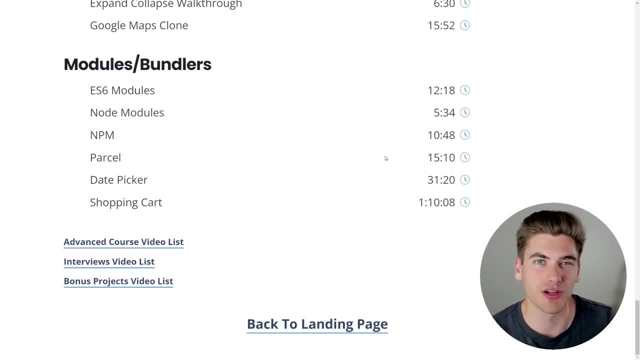 videos and it's a really good idea to try to build out a larger scale project at some point. Don't like make a Facebook clone or something, but make something a little bit bigger than a simple to-do list to really test your abilities and see how you're getting all these concepts. 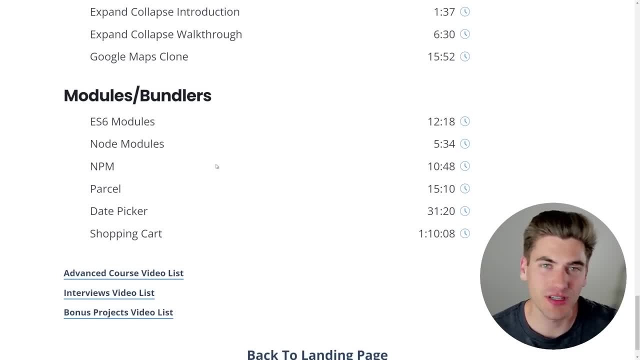 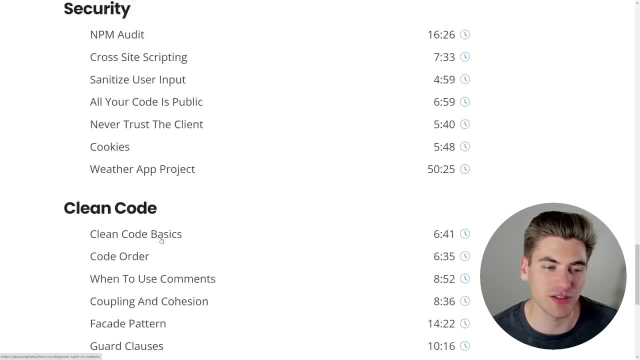 And if they're all clicking for you Now, like I mentioned, that's all the stuff that you need to know in order to become a junior WIP developer. but if you want to take your skills to the next level and kind of become a more intermediate, mid-level developer, this advanced course list. 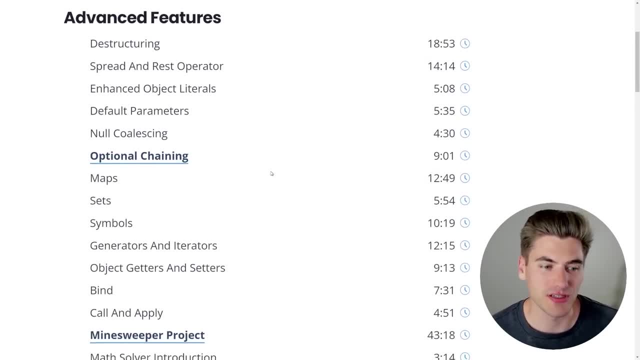 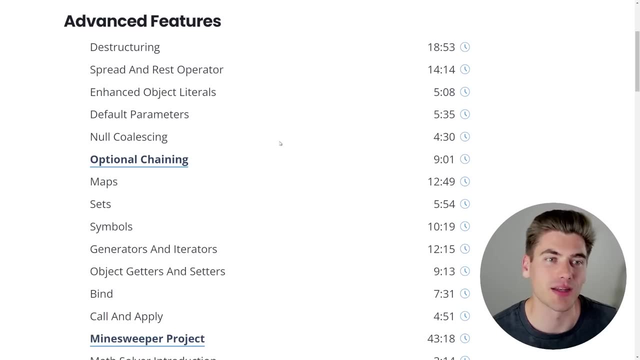 is going to be perfect for you. So if you come into here, the very first thing you'll see is this kind of large section on advanced features. This is just a lot of features that you don't need to know about JavaScript, but are really useful and will save you a lot of time Things. 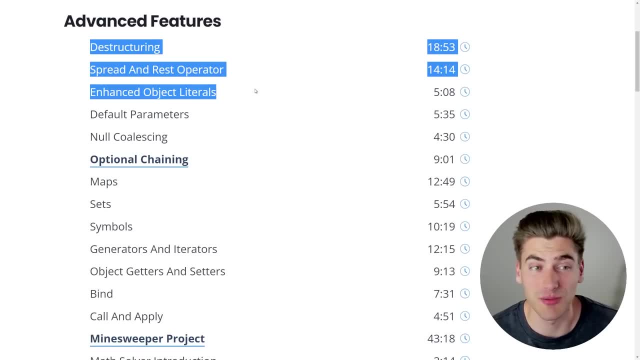 like destructuring the spread and rest operator and how advanced object literals work, default parameters, no coalescing, optional chaining. All of these things are going to help you build your skills and you're going to be able to do a lot of things that you don't need to know. 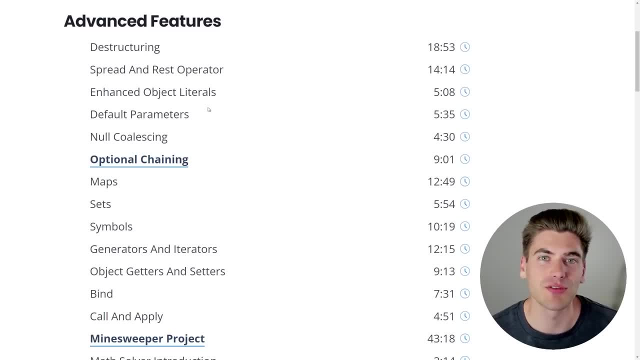 I mean, these features are all pretty new. They were never around when I first learned JavaScript, but they're really important to know Now. I put them in this advanced section just because you don't need them. They're just, you know, syntactical sugar for the most part. 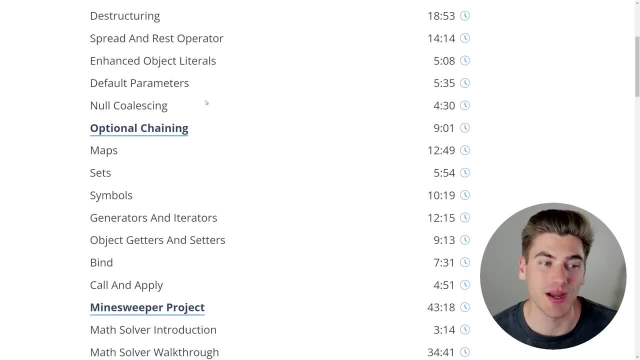 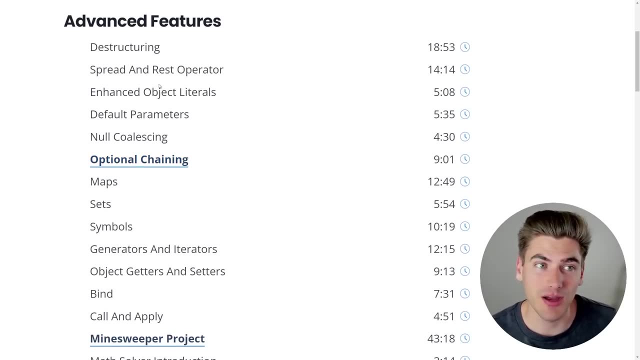 but it does make writing your code a little bit easier and a little bit more enjoyable, So I highly recommend spending your time, look through this section and learn each of these topics. Also, if you're wanting to learn, React everything we've talked about up to this point. 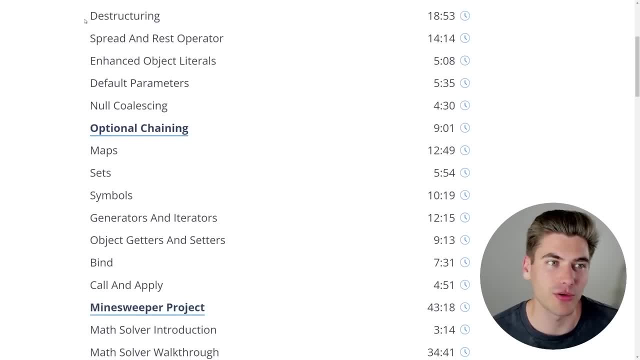 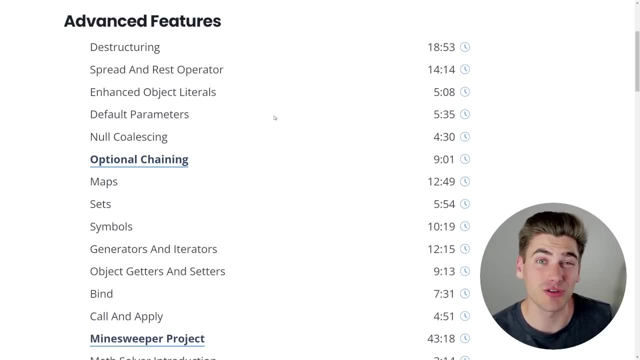 is what I would recommend you learn before you start React. So everything in the beginner course, plus all the things on this advanced features section, those are the concepts I highly recommend learning first before you dive into React. It'll make your journey into React much. 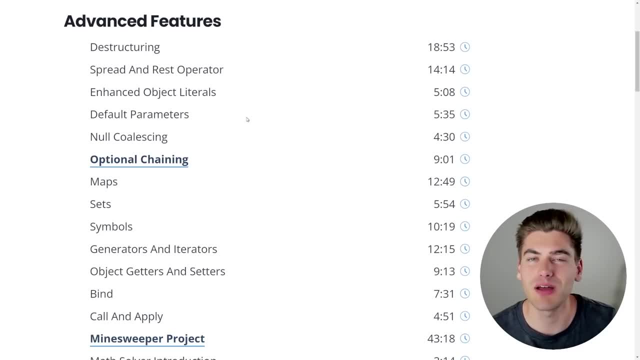 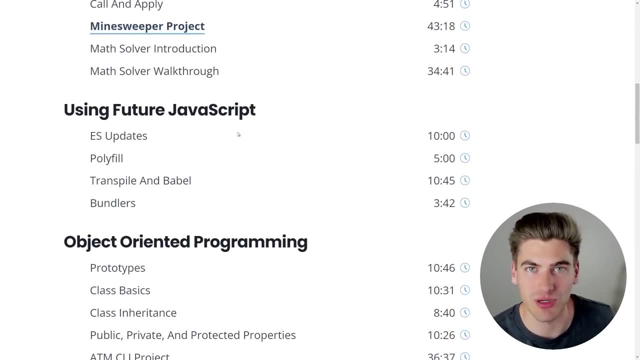 more enjoyable. Now, obviously, you can learn more JavaScript than this, but this is kind of the bare minimum I would recommend you know before you move into React. And the next thing I want to talk about is how you deal with future JavaScript. JavaScript's always changing and there's certain 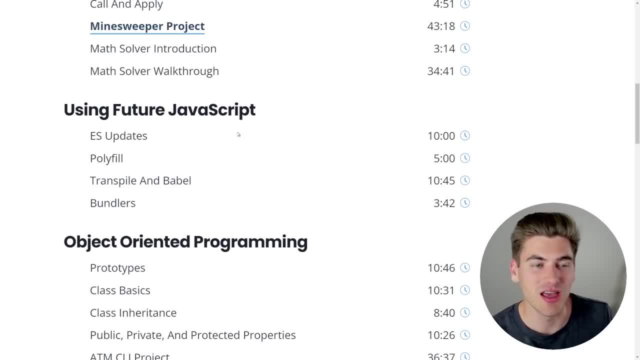 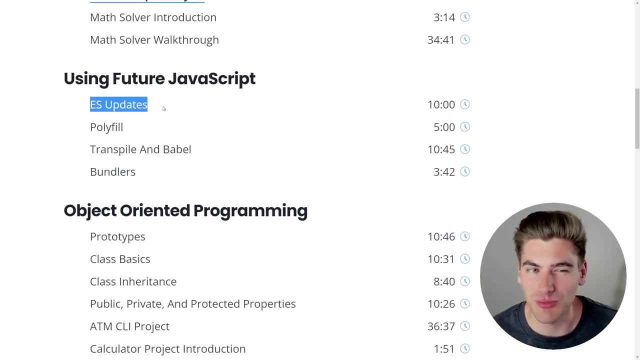 features that are only available in some browsers and not other browsers, and knowing when to use a feature, what features are coming out and if a feature is available, is really important. So I talk about how the actual update process for JavaScript works, how you can actually use 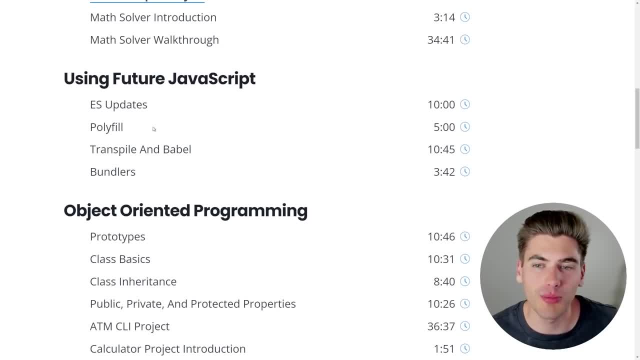 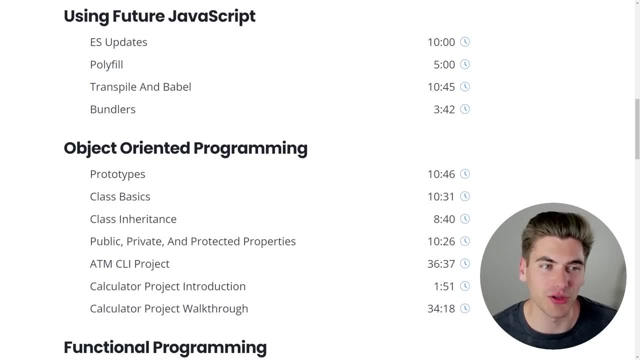 polyfills to use features that are only available in some browsers and all browsers, and how things like transpiling with Babel work in order to actually make your JavaScript work on every browser. and then, finally, a little bit more on bundlers like Parcel and Vite. Now the next two. 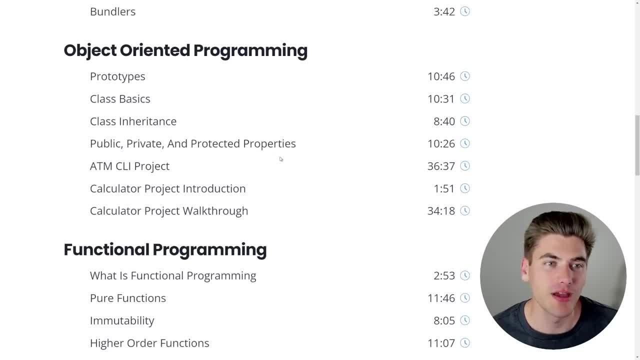 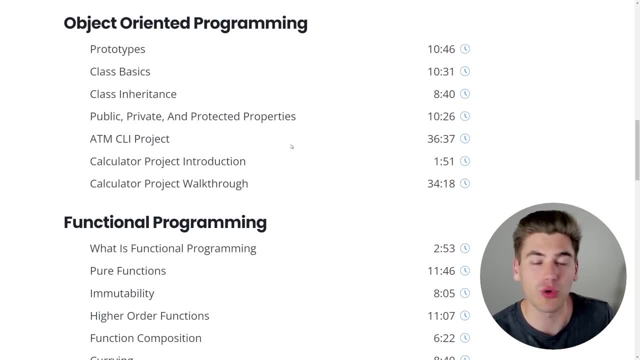 sections of this course. we have object-oriented programming and functional programming. These are two different programming paradigms, essentially just two different ways to program. Object-oriented programming, I would say, is a little bit of an older way of doing it. It's not that it's outdated. 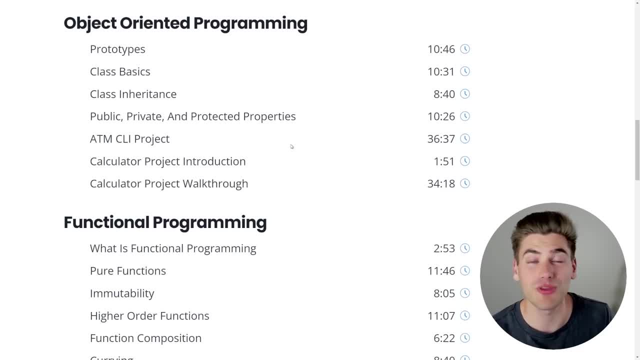 it just came first. It's not that it's outdated. it's not that it's outdated. it just came first For the most part and it was popularized a lot more with things like Java became very popular. So object-oriented programming is when you use classes and class-based programming. 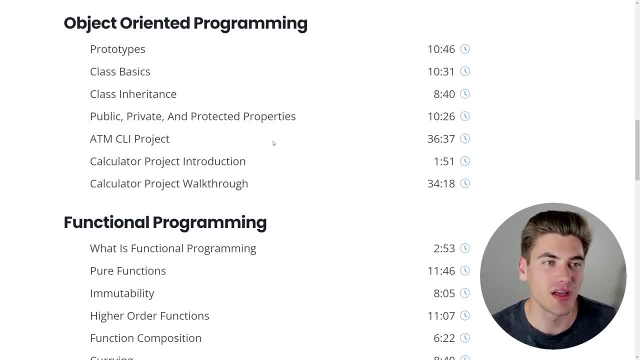 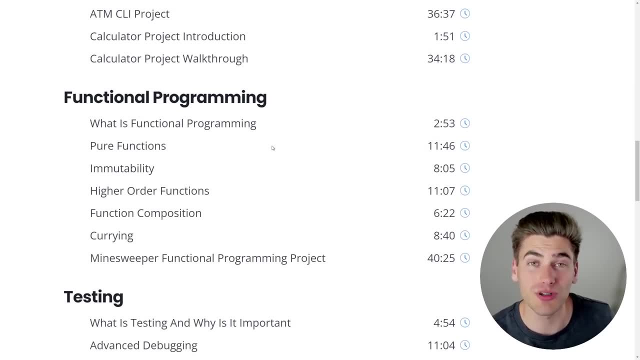 and it has its own place and is definitely useful in particular projects. but I find that JavaScript doesn't lend itself as well to object-oriented programming and instead a more functional programming approach, I think, works a little bit better for JavaScript. I think it's still really. 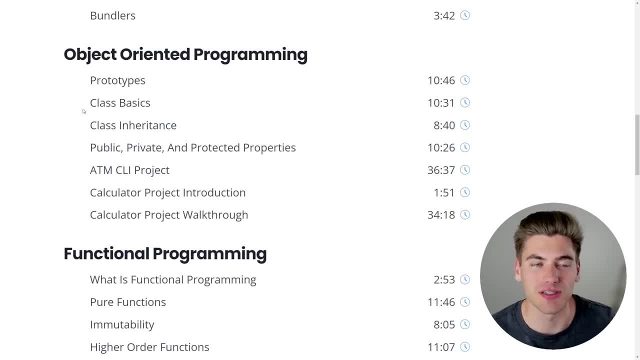 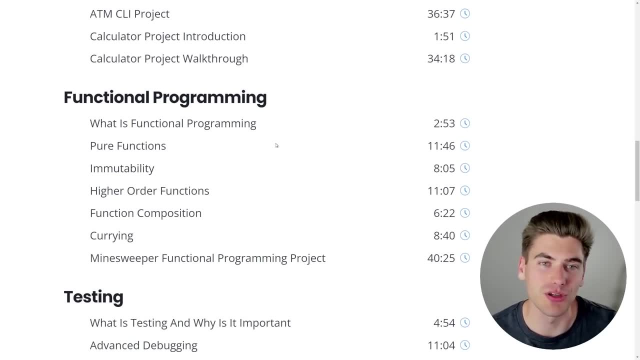 important to learn both of them: understand how classes work and how inheritance works in object-oriented programming, and also understand how things like immutability and pure functions work in functional programming, because if you want to write really good code, most likely you're going to be writing somewhat of a combination of both of them. 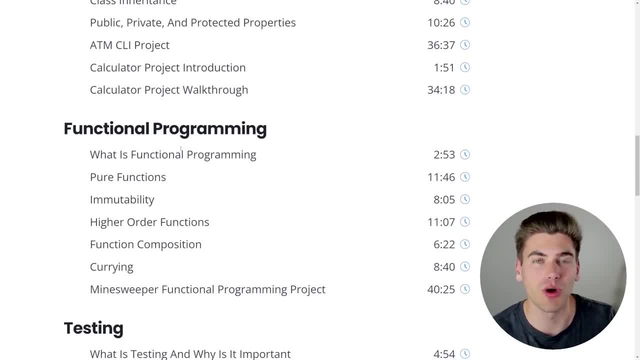 I generally lean slightly more towards functional programming, but depending on what you're actually building out and how you enjoy programming, you may lean towards one way or the other. so it's important to understand the pros and cons of both and how they both work. 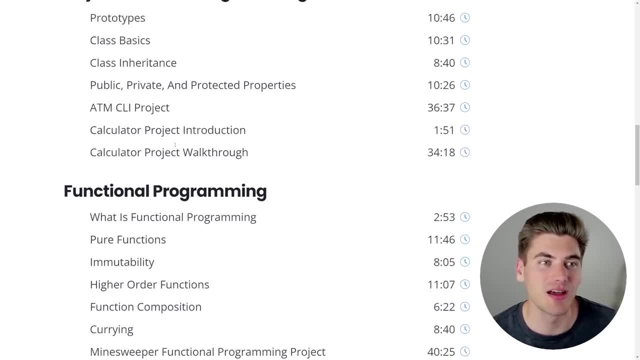 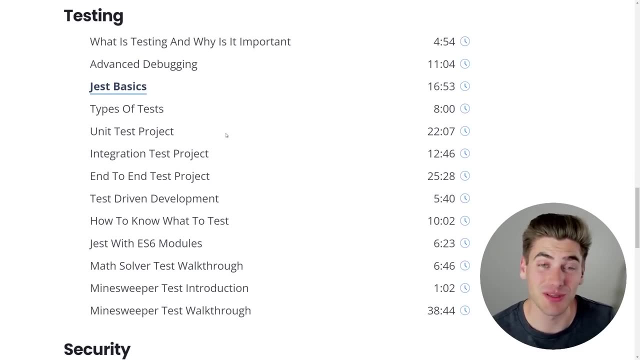 and these two sections just cover the main concepts you need to understand about object-oriented programming and functional programming. Now the next big section you'll see here is a quite large section on testing. This is something most developers don't even cover at all when they're learning, but having some testing knowledge before you apply for your first job. 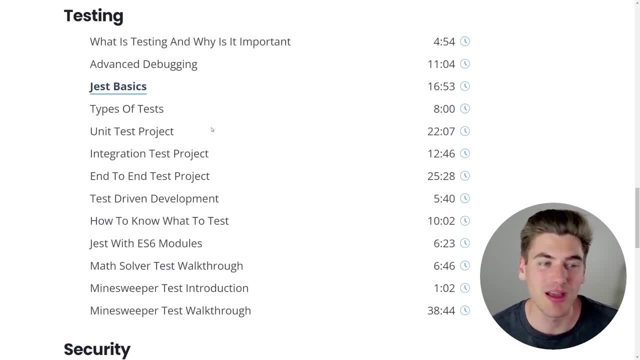 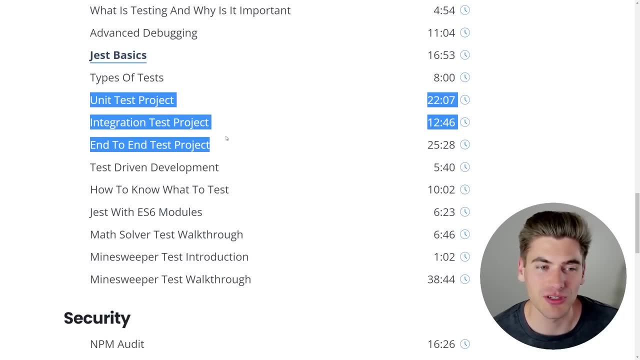 is crucial because it's going to make you stand out above most other people, and the real important thing about testing is just practice testing. You'll notice in this section of the actual thing here, I have three different projects here for testing each different type of test, and at the bottom I have even more projects on how to test. 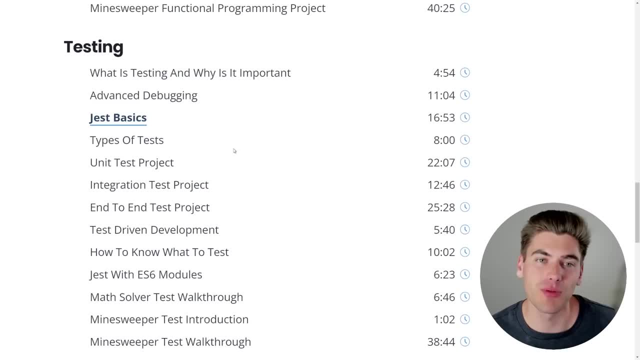 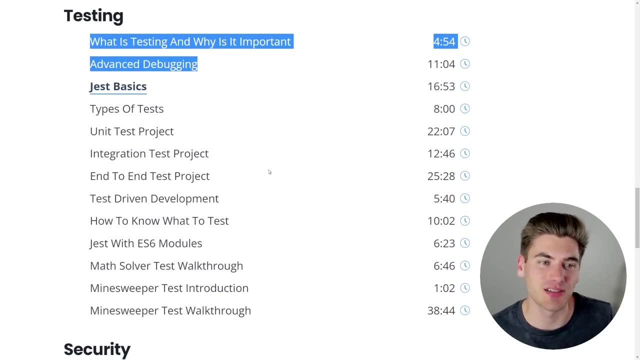 everything. Over half of this section is just on projects implementing testing. so it's important to understand kind of what testing is, why to test what you should test. but really to understand how to test and what to test, you just need to practice over and over again. 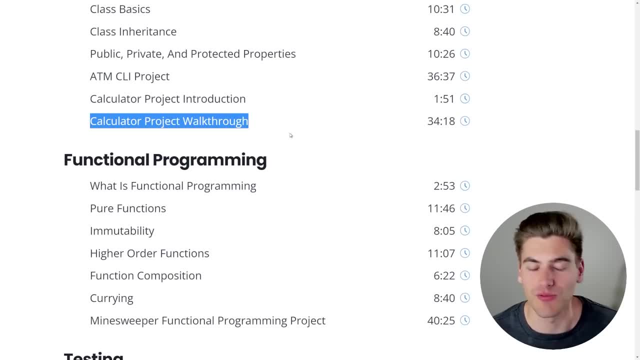 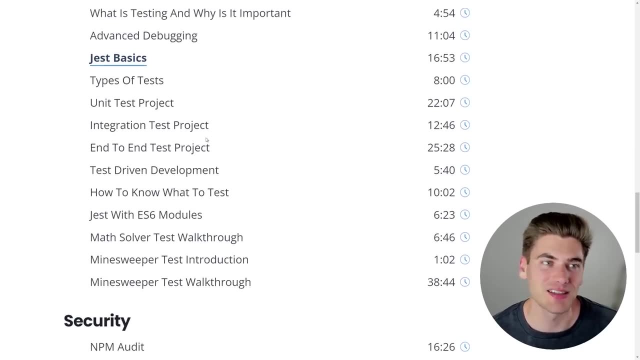 So take some of the projects you built previously inside of this- whatever projects you decided- and just try adding tests to them. whether they're unit tests, integration tests, end-to-end tests, it doesn't matter. just try adding these tests in and seeing what you can. 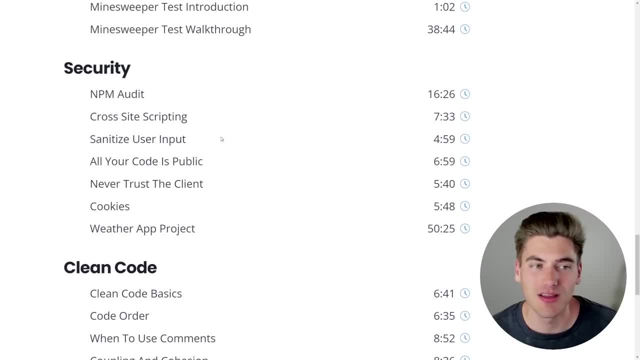 learn and seeing how it works. that's really the best way to do this. Now the next and almost final step here we have is security. Security is really important because you want to make sure you don't leak sensitive API keys. you don't want to expose user passwords. 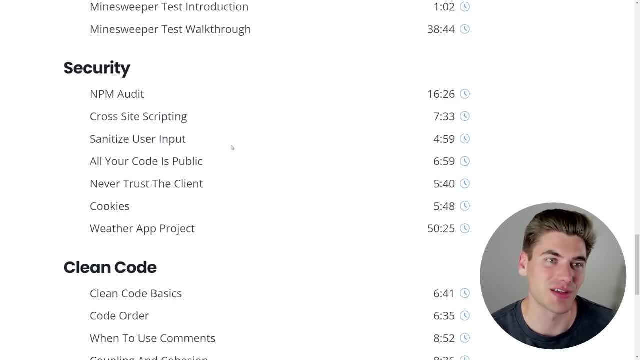 and that kind of stuff. so this covers some of the more basic concepts of security. The course is a little bit more focused on front-end JavaScript and this roadmap itself is more focused on front-end JavaScript, so I don't have as much back-end related security stuff. 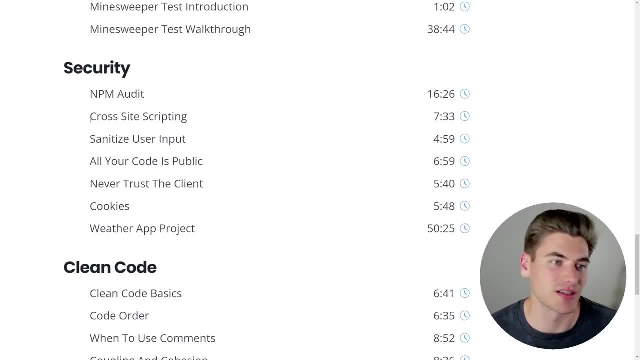 but there are some back-end related stuff in here as well as how to handle different things like cross-site scripting, sanitizing, user input and stuff like that. It's mostly high-level stuff, but it's still really important and gives you a good groundwork for how to do security in an. 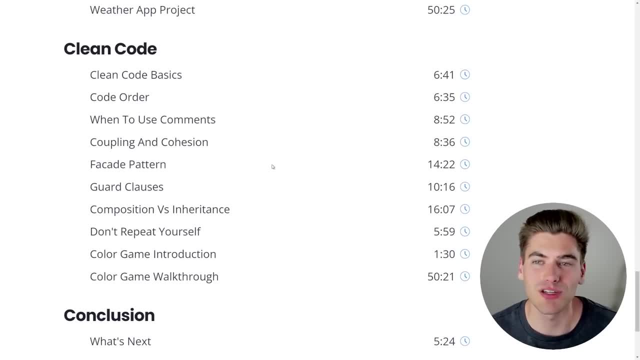 application. Now, the final section that we have here is the clean code section, and this is somewhat opinionated, but it really helps you to understand how to actually write better code, because anybody can write a code for a project and it's really important to understand how to. 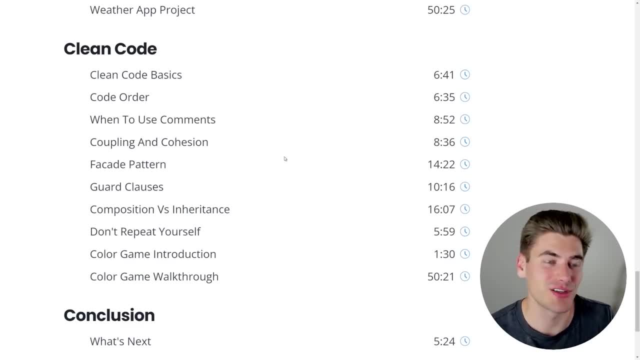 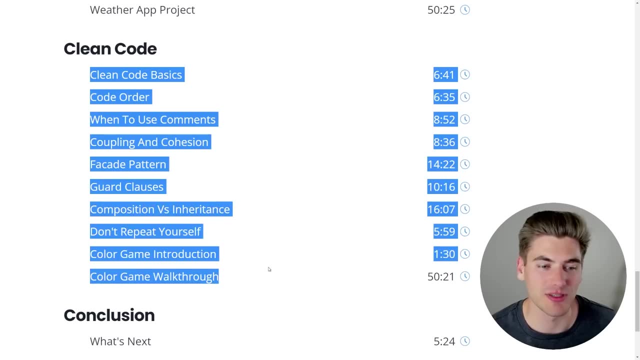 project. but not everyone can write good clean code for projects. So this kind of gives you some basic ideas of how you can go about implementing cleaner code in your projects. Obviously, not all of these things are going to be something you want to implement, but it just kind of gives you the 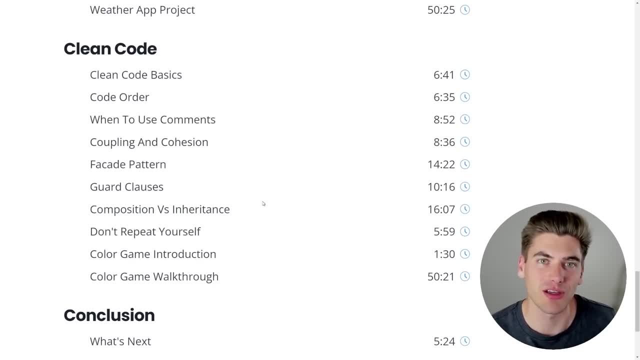 starting point of things to think about in order to actually write good, clean code- which is one of the most important steps to go from a junior developer to an intermediate, mid-level developer- is learning how to write cleaner, better code. Now, once you learn all of those different concepts, 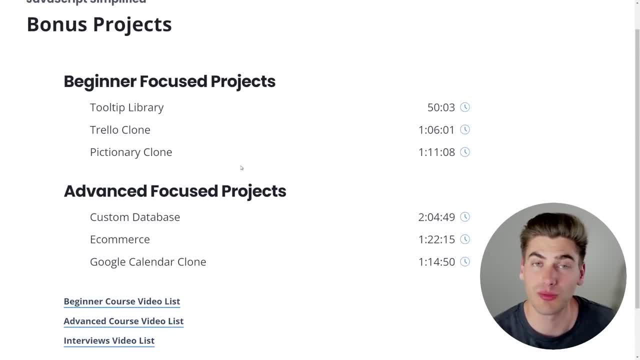 you can see, I have this bonus project section. This just has some kind of larger projects that you can build. You can use these projects if you want or you can build your own projects, but I recommend going ahead and trying to build out some larger scale projects. 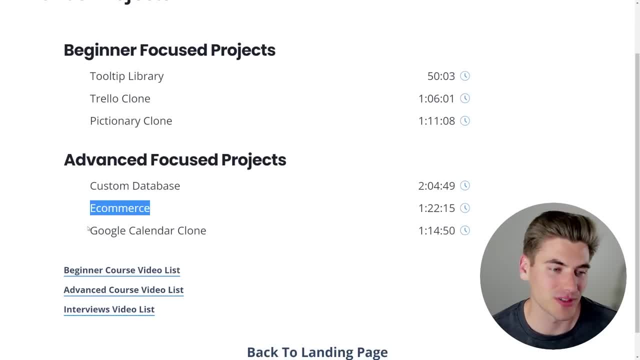 You can see that we have things like building out a custom database, a full ecommerce site, google calendar clone. These are larger scale projects and these should take you a significant amount of time. I would say a minimum amount of time would be one week on these projects. maybe up to a maximum of about two months. I wouldn't really want to do a project much longer than that, at least if you're trying to do multiple projects. but you can also do one large project that's going to take you maybe three or four months long. 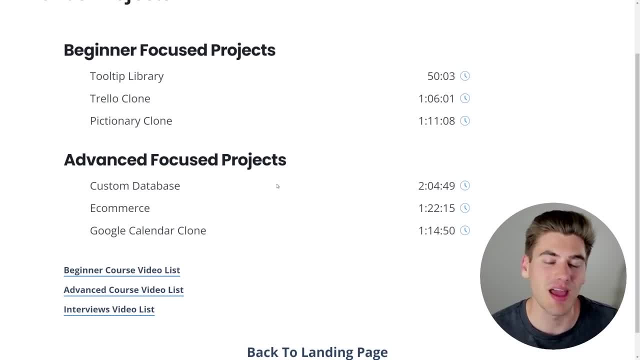 This is the point where you can actually do that, because you have all of the knowledge you need, and it's the best way to practice things like writing clean code, because you don't really notice bad code unless it's in a larger project you're working on for an extended period of time. 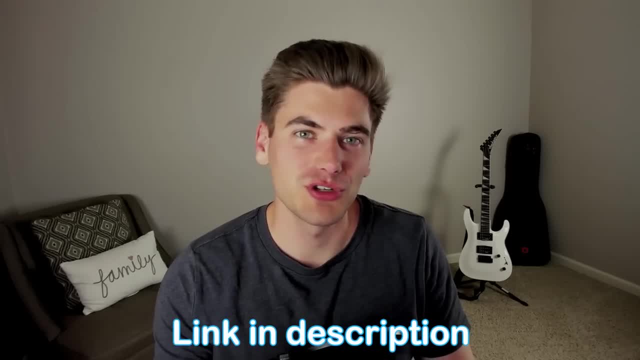 So if you're interested in checking out this roadmap, I'm going to have it linked down in the description. You can go ahead and look at it, watch some of the demo videos and if you want to take my course that exactly follows this roadmap, I'm also going to have 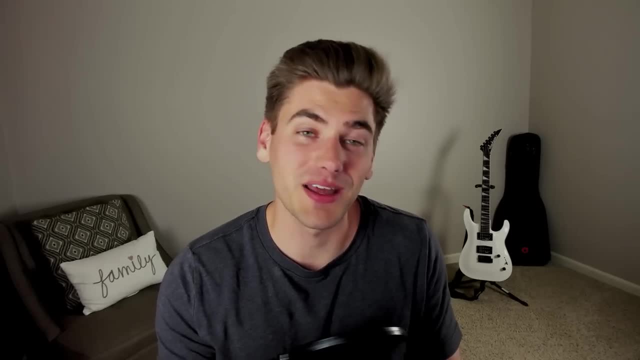 that linked down in the description. I think it's one of the best ways to learn JavaScript, but I am slightly biased With that. said, thank you very much for watching and have a good day.